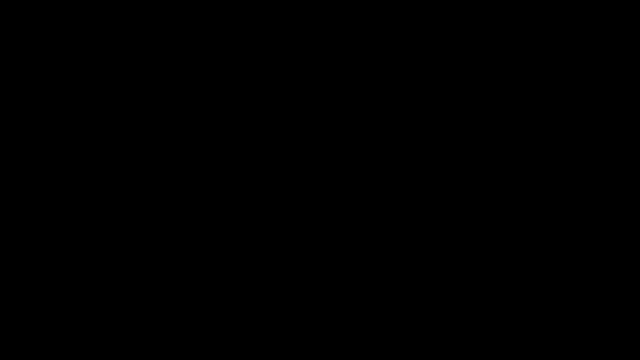 Now in this lesson we're going to talk about graphing quadratic functions in vertex form without using a data table. So let's start with this example: x minus 2, squared minus 3.. First, find a vertex. We can see that it's positive 2 and negative 3.. 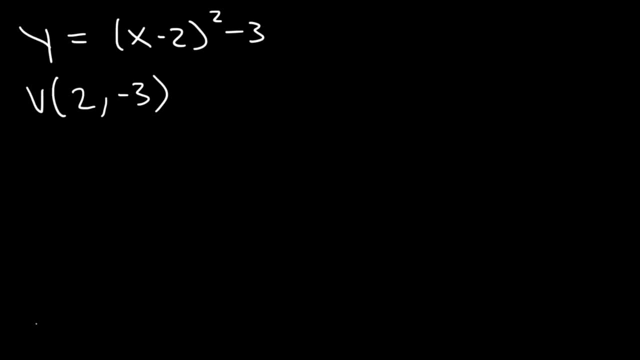 Change this sign, but don't change this one. Now let's go ahead and plot the vertex. So it's 2 units to the right and down 3, so it's over here. Now. the parent function is: y is equal to x squared. 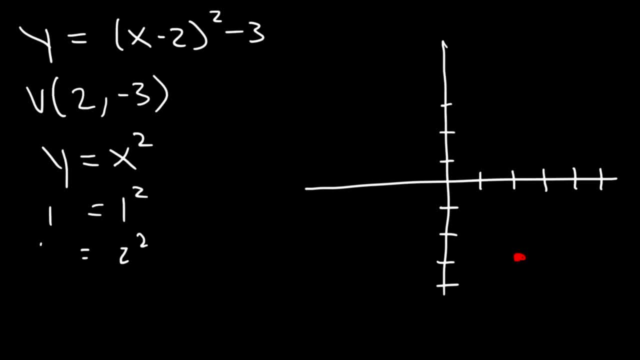 1 squared is 1, 2 squared is 4.. Why am I telling you this? Well, it turns out that as you travel 1 unit to the right- the next point- you can find it by going up 1.. 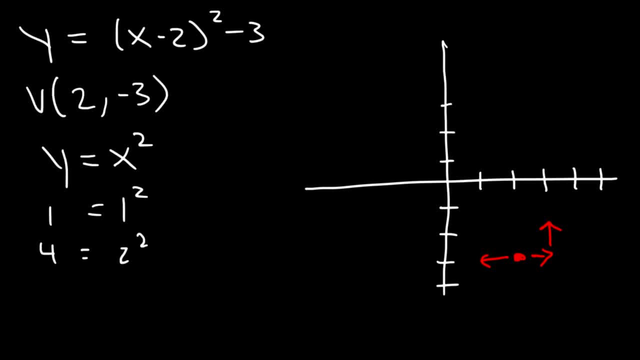 And as you travel 1 to the left, go up 1, that will give you the next point. So the next point is that we have one at 3, negative 2, and also 1, negative 2.. Now, based on this, as you travel 2 units to the right from the vertex to get the next point, go up by 4 units. 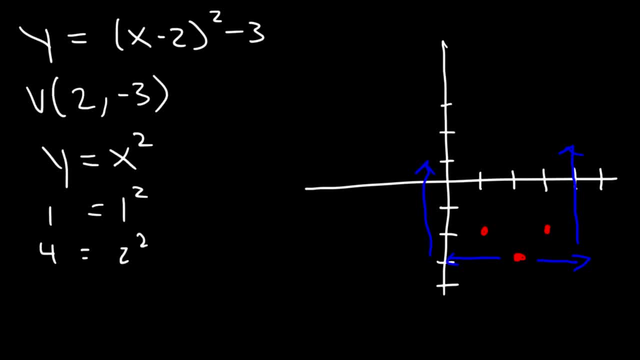 And as you travel, 2 units to the left go up by 4.. So on the right side it will take us to the point 4, 1. And on the left side we're going to have the point 0, 1.. 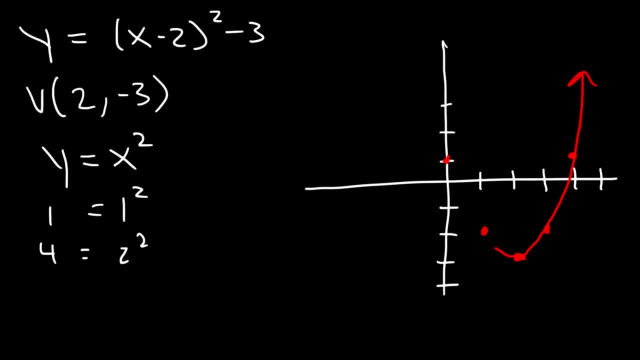 And now we can graph it, So we can see that the domain is going to be everything, all real numbers, from negative infinity to infinity. The lowest y value is negative 3,, the highest is infinity. So the range is from negative 3 to infinity, including negative 3.. 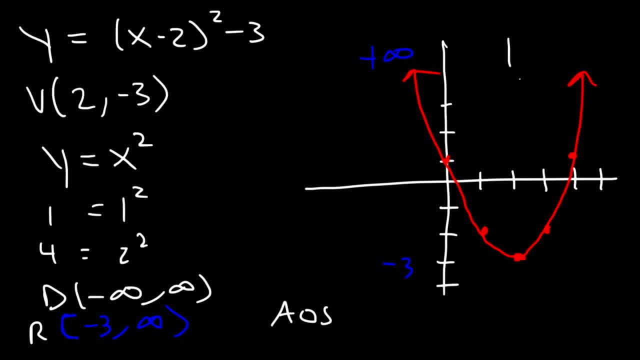 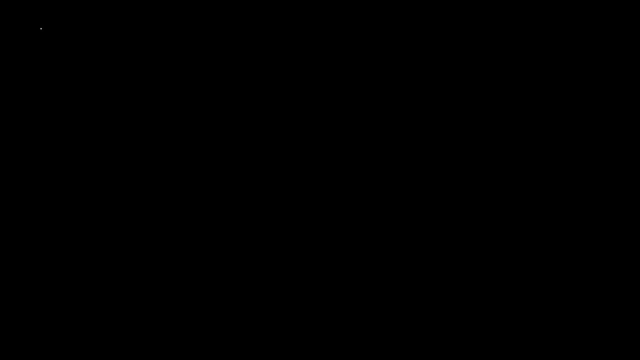 The axis of symmetry, that's going to be the x coordinate of the vertex, Which is x equals 2.. And because it opens upward, we have a minimum value of negative 3.. Let's try another example: Negative 2 times x plus 1, squared minus 5.. 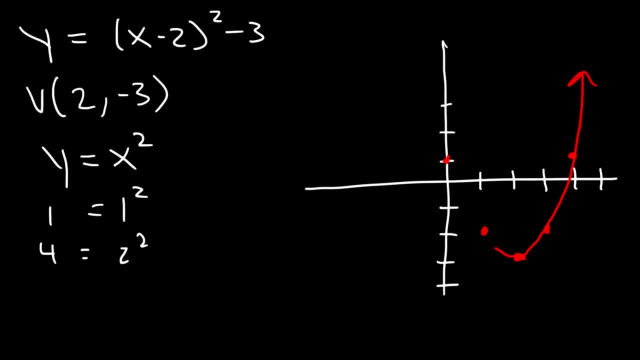 And now we can graph it, So we can see that the domain is going to be everything, all real numbers, from negative infinity to infinity. The lowest y value is negative 3,, the highest is infinity. So the range is from negative 3 to infinity, including negative 3.. 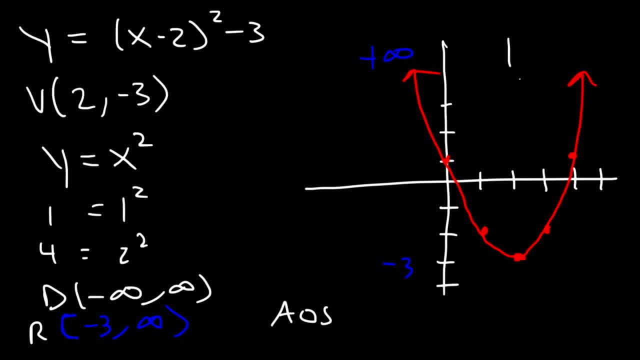 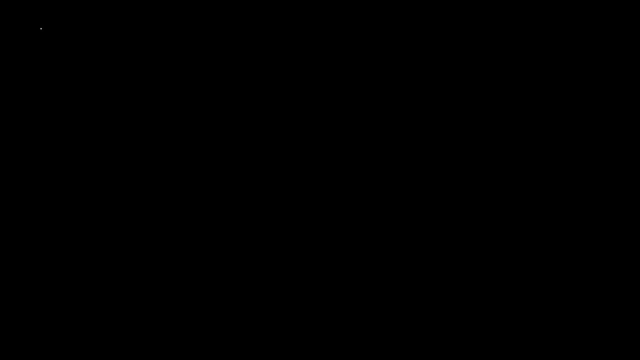 The axis of symmetry, that's going to be the x coordinate of the vertex, Which is x equals 2.. And because it opens upward, we have a minimum value of negative 3.. Let's try another example: Negative 2 times x plus 1, squared minus 5.. 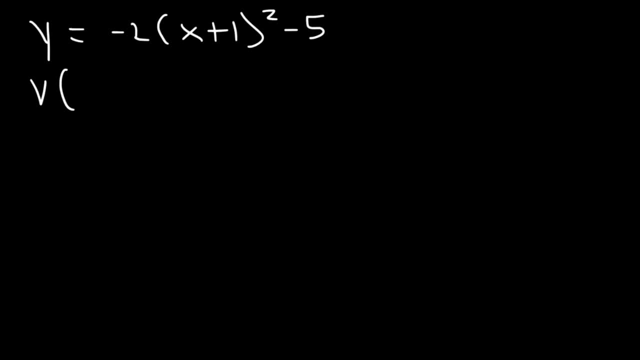 So first find the vertex and then graph it. Okay, Determine the axis of symmetry domain and range everything. The vertex is negative 1, negative 5.. Change positive 1 to negative 1, but don't change negative 5.. 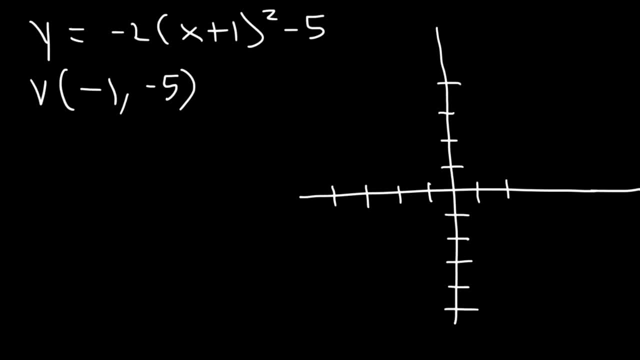 Negative 1, negative 5 is over here Now. notice that we have a 2 in front. Let's make it positive 2.. If we make it negative 2, it's going to open downward and it's not going to be enough space to graph it. 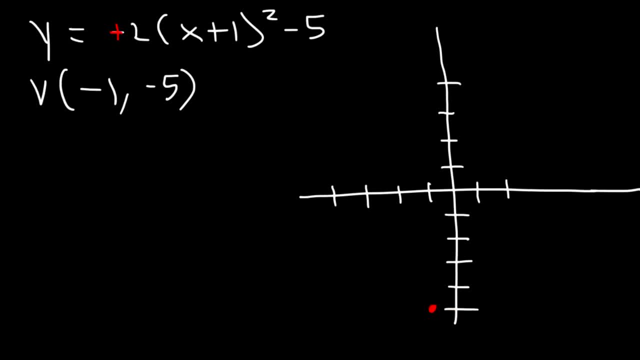 So let's change it to positive 2.. How can we find the next point? The parent function is 2x squared As opposed to 1x squared. So 2 times 1 squared it's not going to be 1, it's going to be 2.. 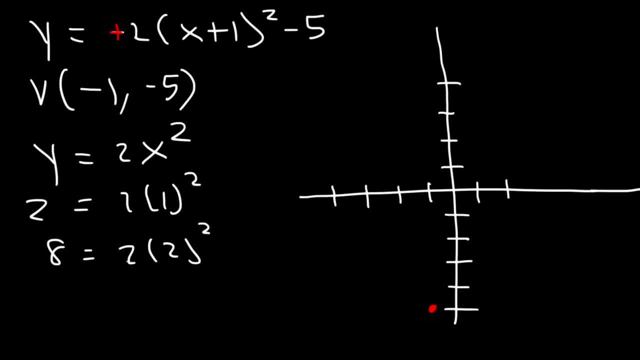 And 2 times 2 squared is 8.. So, as we travel 1 unit to the right, instead of going up 1, we need to go up 2 units. So the next point is going to be 0, negative 3.. 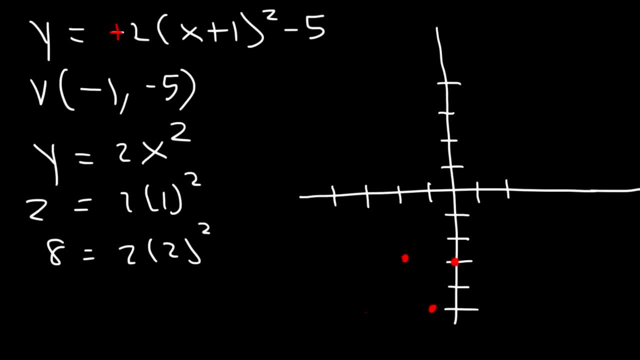 And the same is true for the left side. It's going to be negative 2, negative 3.. Now, when we plug in 2, it's going to be negative 3.. When we plug in 2 for x, we're going to get 8.. 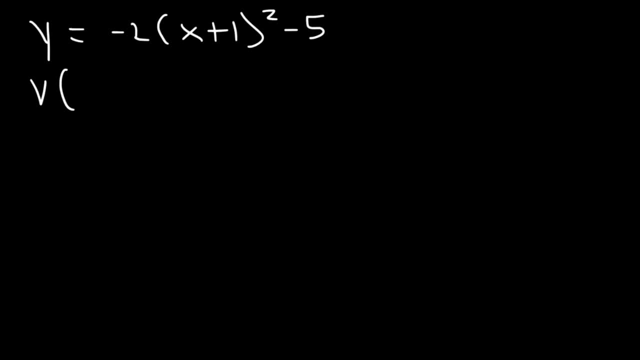 So first find the vertex and then graph it. Okay, Determine the axis of symmetry domain and range everything. The vertex is negative 1, negative 5.. Change positive 1 to negative 1, but don't change negative 5.. 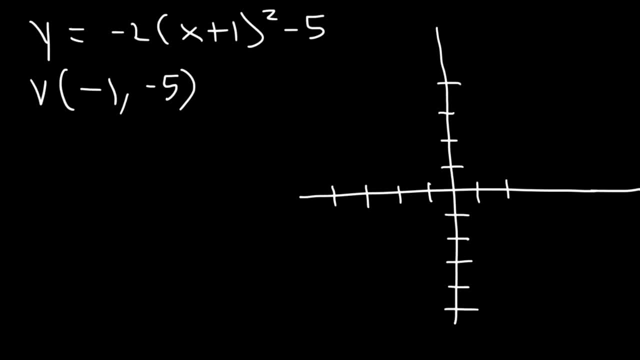 Negative 1, negative 5 is over here Now. notice that we have a 2 in front. Let's make it positive 2.. If we make it negative 2, it's going to open downward and it's not going to be enough space to graph it. 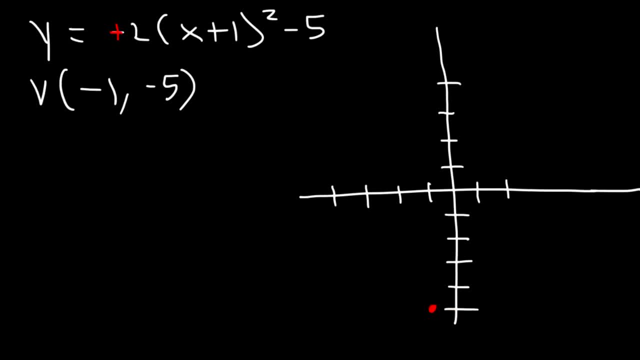 So let's change it to positive 2.. How can we find the next point? The parent function is 2x squared As opposed to 1x squared. So 2 times 1 squared it's not going to be 1, it's going to be 2.. 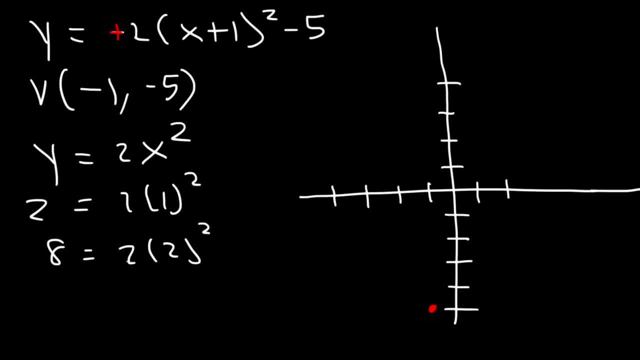 And 2 times 2 squared is 8.. So, as we travel 1 unit to the right, instead of going up 1, we need to go up 2 units. So the next point is going to be 0, negative 3.. 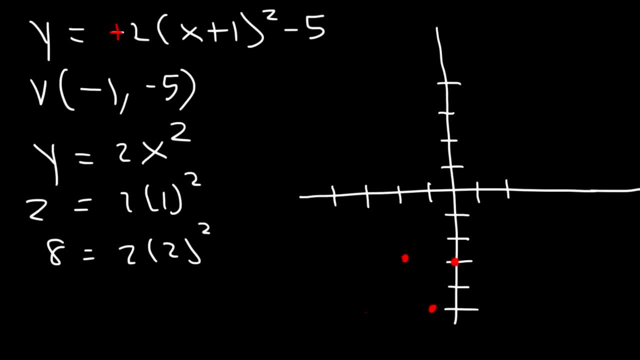 And the same is true for the left side. It's going to be negative 2, negative 3.. Now, when we plug in 2, it's going to be negative 3.. When we plug in 2 for x, we're going to get 8.. 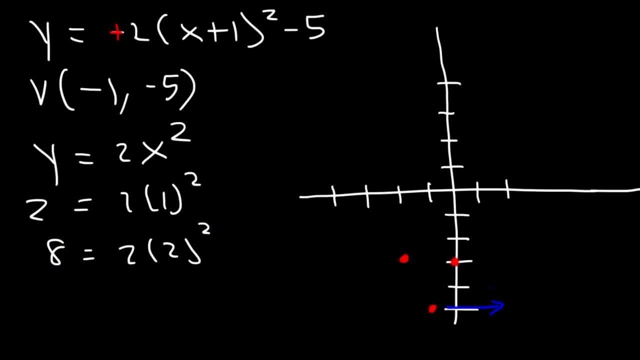 So, as we travel 2 units to the right, we need to go up 8 units, which will take us to positive 3.. And as we travel 2 to the left, we need to go up 8 units. So this will give us the point 1, 3, and negative 3, 3.. 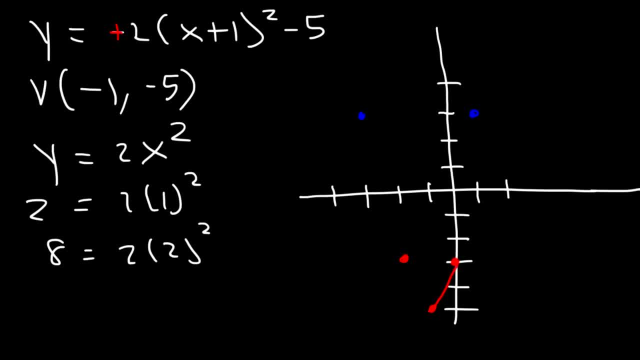 So now let's graph it. So we're going to have a graph that looks like this: The domain is going to be the same thing, all real numbers. We can see that the lowest y value is negative 5,. the highest is infinity. 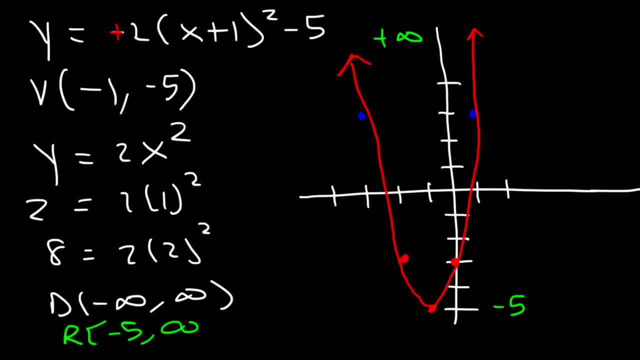 So, therefore, the range is from negative 5 to infinity, And since it opens upward, the minimum value is negative 5.. And the axis of symmetry will always be the x coordinate of the vertex, So that's x equals negative 1.. 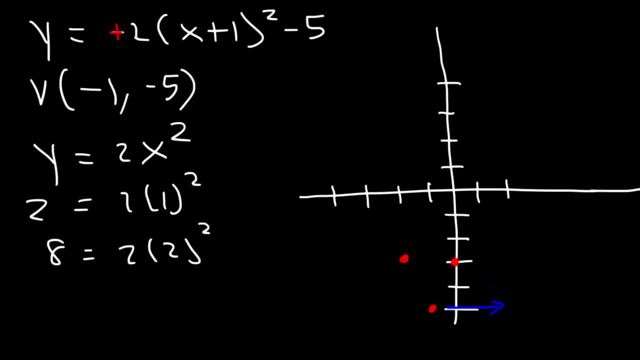 So, as we travel 2 units to the right, we need to go up 8 units, which will take us to positive 3.. And as we travel 2 to the left, we need to go up 8 units. So this will give us the point 1, 3, and negative 3, 3.. 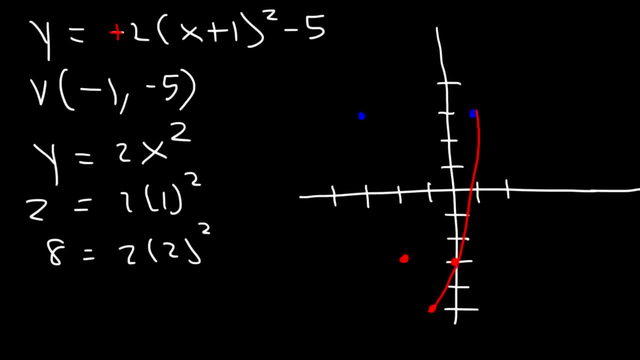 So now let's graph it. So we're going to have a graph that looks like this: The domain is going to be the same thing, all real numbers. We can see that the lowest y value is negative 5,. the highest is infinity. 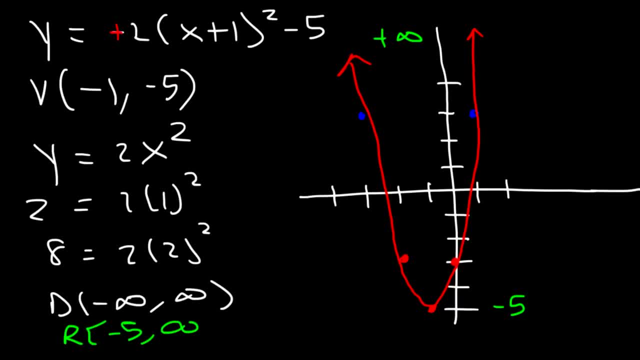 So, therefore, the range is from negative 5 to infinity. And since it opens upward, the minimum value is negative 5.. And the axis of symmetry will always be the x coordinate of the vertex. So that's, x equals negative 1. That's the AOS. 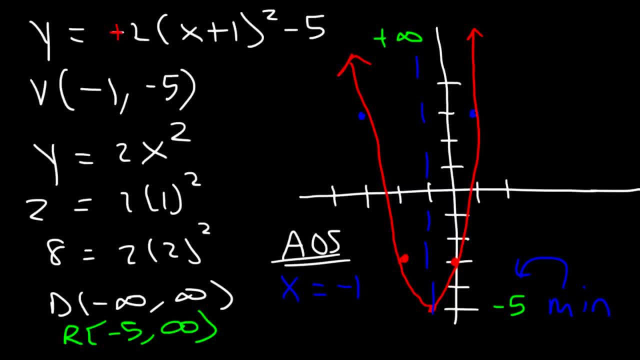 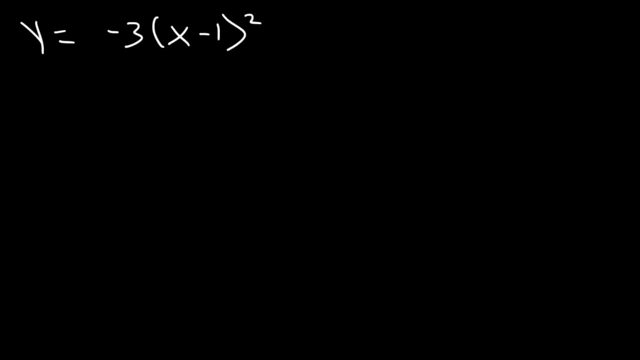 Let's try one more example: Negative 3, x minus 1, squared plus 9.. So go ahead and find the vertex and everything else. The vertex is: The majority of the graph is going to be above the x axis And I need more space. 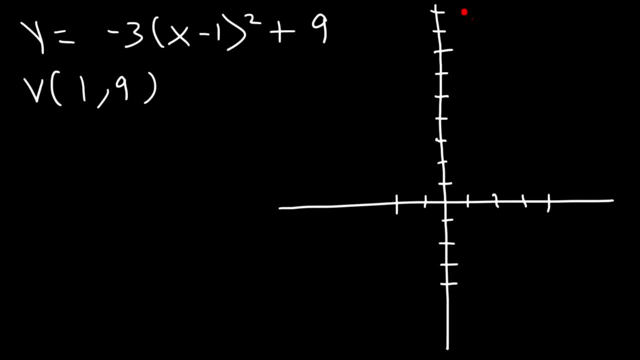 So let's plot the point Now. notice that we have a negative 3.. If we plug in 1,, y will change by negative 3.. If we plug in 2,, 2 squared is 4, times negative 3.. 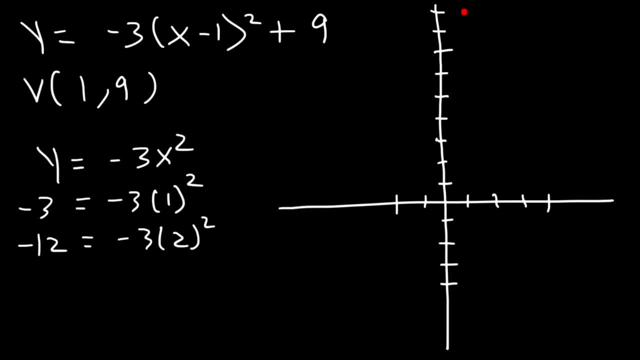 The y value will change by negative 12.. So as we travel one unit to the right, we need to go down 3 units, And the same is true as we go to the left, We need to go down 3.. So this will give us the point. 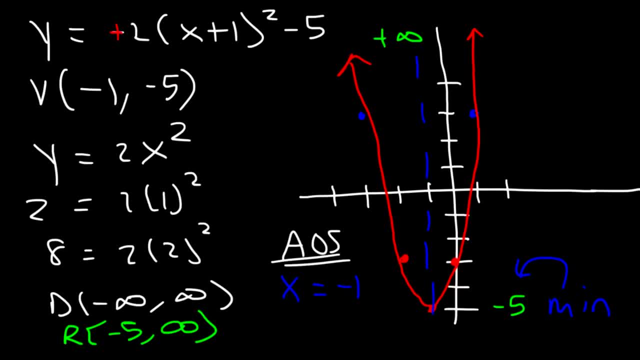 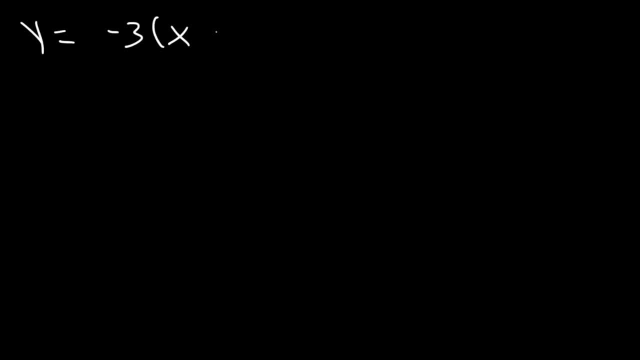 That's the AOS. Let's try one more example: Negative 3, x minus 1, squared plus 9.. So go ahead and find the vertex and everything else. The vertex is: The majority of the graph is going to be above the x axis. 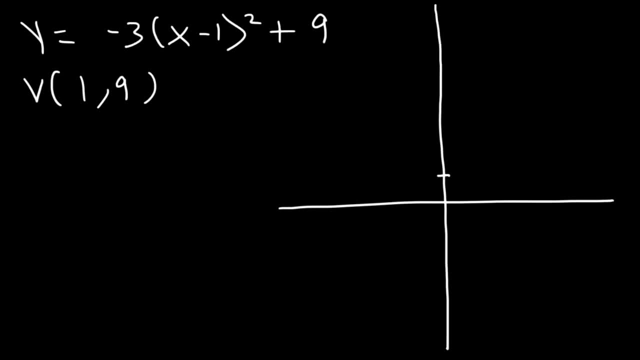 And I need more space. So let's plot the point 1, 9.. Now notice that we have a negative 3.. If we plug in 1,, y will change by negative 3.. If we plug in 2,, 2 squared is 4, times negative 3.. 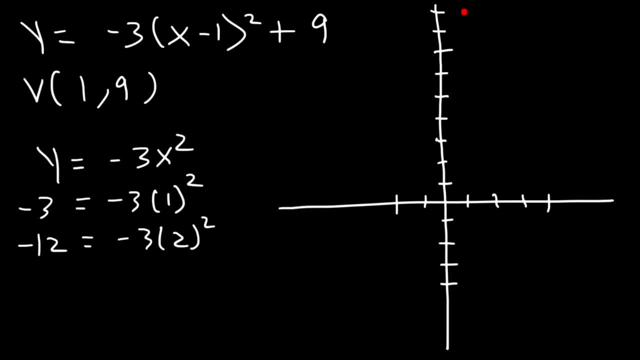 The y value will change by negative 12.. So as we travel one unit to the right, we need to go down 3 units, And the same is true as we go to the left, We need to go down 3.. So this will give us the point. 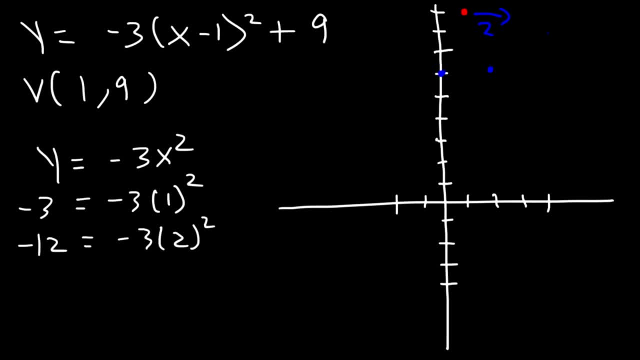 Now, as we travel 2 units to the right, we need to go down 12 units, Which will take us to negative 3.. And the same is true for the left side: As we travel 2 units to the left, we need to go down 12 units. 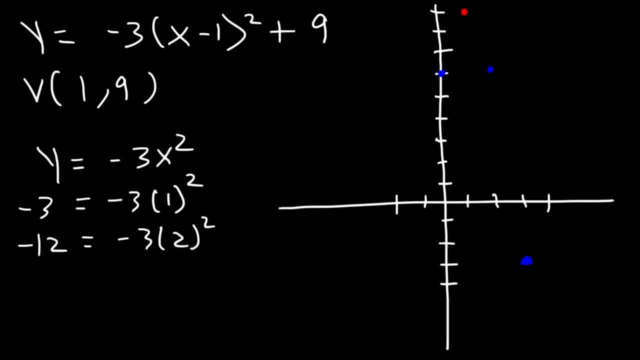 So this will take us to the point Because 9 minus 12 is negative 3. And 2 to the left will take us to an x value of negative 1. And then down to negative 3 as well, And so the graph is going to look something like this: 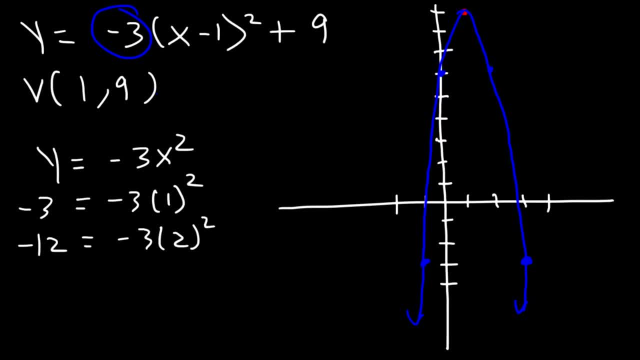 As you can see, as we increase the a value, the graph becomes more narrow. It stretches vertically. The domain is still all real numbers. The highest y value is 9.. The lowest is negative infinity. So therefore the range is from low to high, negative infinity to positive 9..